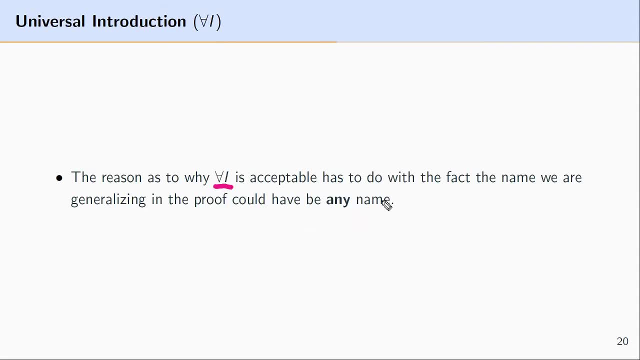 The reason why universal introduction is acceptable has to do with the fact that the name we generalize or that we turn into a universally quantified variable could be any name. That is when we're reasoning from PA to for all, X, PX. 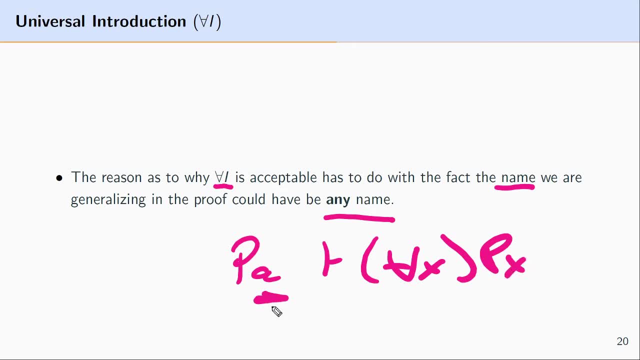 this name has to have special properties, It has to meet certain conditions, And the general condition is that this name could have been B or C or D or E or any name, And since that it could be any name, that is, since this name could refer to any item in our domain. 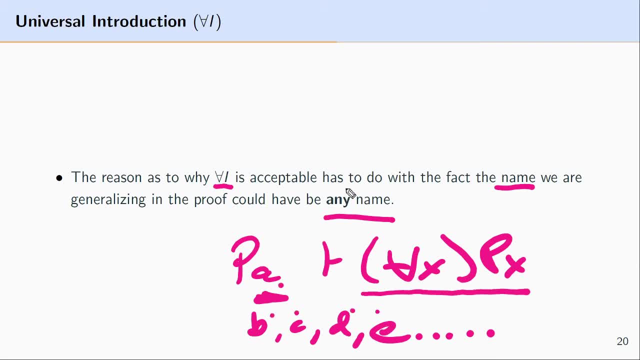 this allows us to generalize. So one of the reasons that universal introduction is acceptable has to do with certain restrictions we place on when you can use universal introduction, And the core of that restriction has to do with the fact that the name that we universalize is arbitrary. 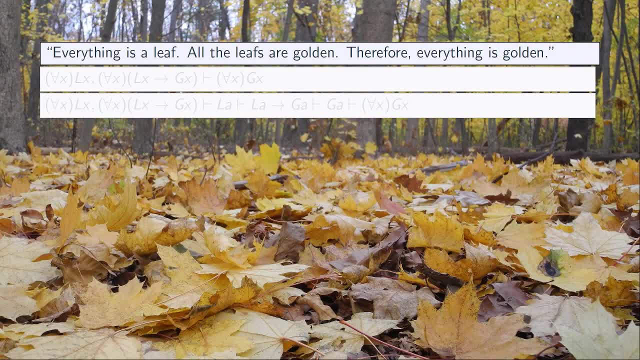 Let's look at an example of this in the context of a proof. Suppose we're talking about a domain and I say everything is a leaf, And then I also say all leaves, or all the leaves are golden. Therefore, everything is golden. 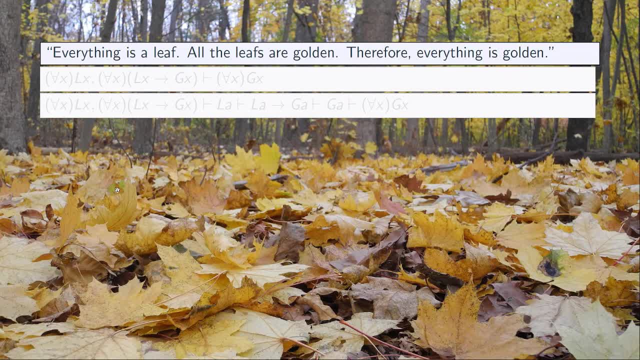 This looks like a valid argument and we might represent this as follows: For everything is a leaf, we could write for all x, l, x. For all of the leaves are golden, we can write a x, l, x, then g x. 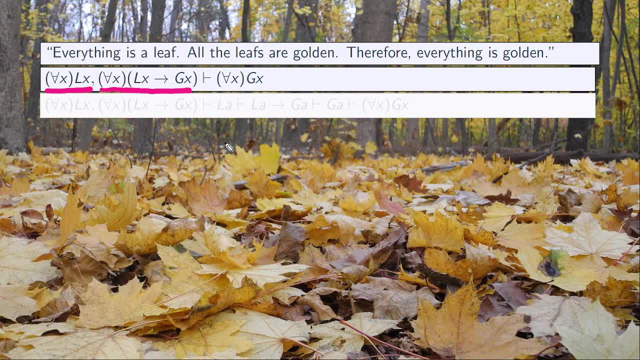 And for everything is golden. we would write the universal quantifier a x, g, x. In the context of a proof, we would reason as follows: First we have the premises a x, everything is a leaf. 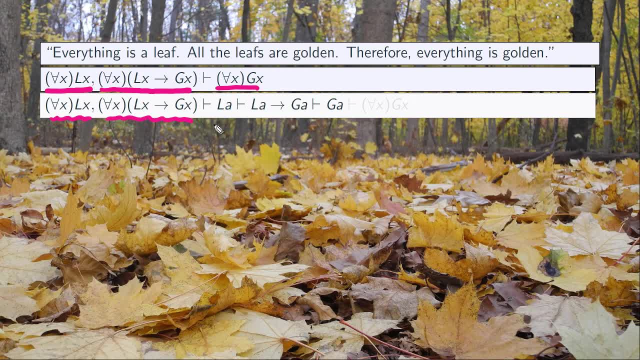 a, x, l, x, then g x. All of the leaves are golden, And then we could reason from a x, l, x to l? a, using universal elimination. We're reasoning from: everything is a leaf. 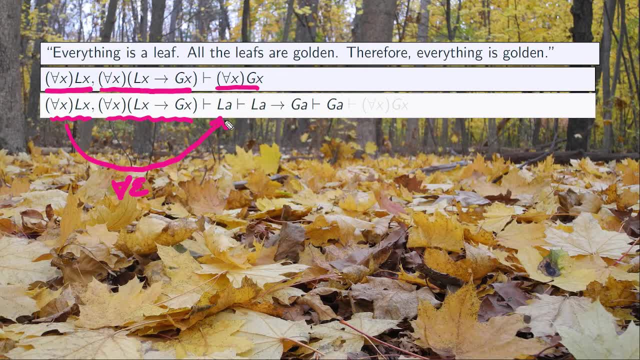 to a named leaf that we name with a is a leaf, And also from a x, l x, then g x. the second premise: we could reason using universal elimination If a particular item is a leaf. 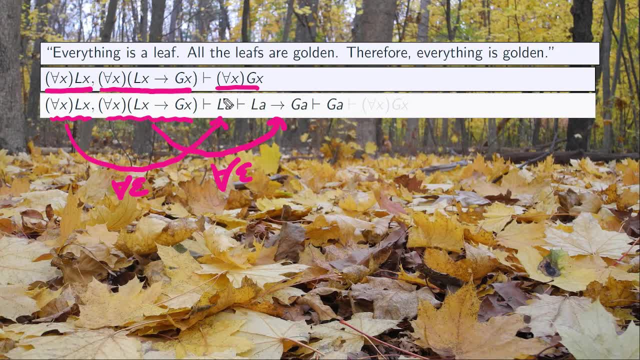 then that particular item is golden. Next, from the fact that we have a particular item that we named, a is a leaf, and we said that if a, that thing is a leaf, then it's golden. we could reason to. 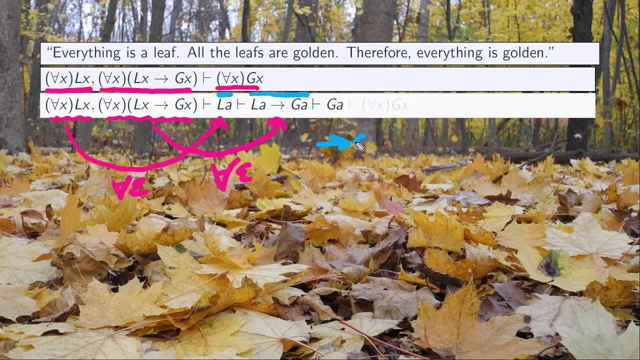 using conditional elimination, also known as modus ponens to that item is golden. Now the last step here is the use of universal introduction. That is, we want to know whether or not it's acceptable to reason from a particular item. 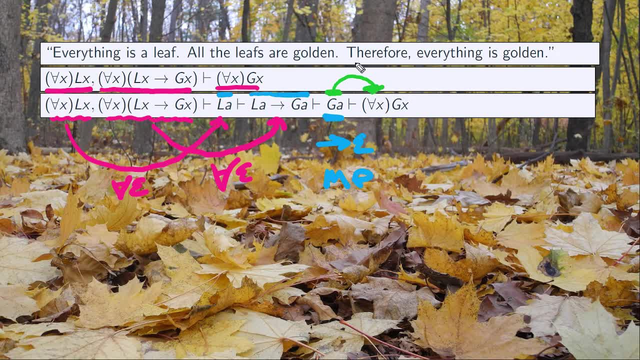 being golden to everything is golden, Like in our example up here. we reason to everything is golden. One of the reasons that we might say that this is acceptable, that in this instance it's acceptable to use universal introduction replacing the name a. 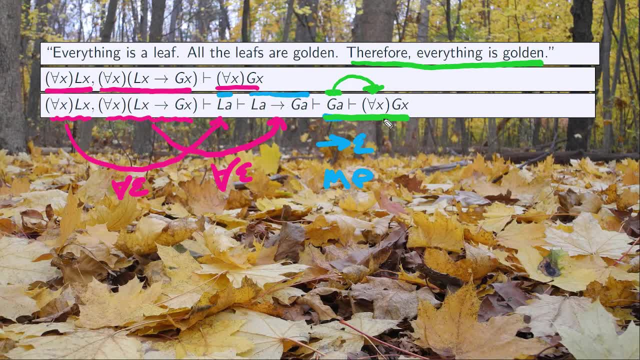 with a universally quantified variable, x is because that this a here could have been b, it could have been c, it could have been d, it could be any name that refers to any item in the domain, And the reason for that is: 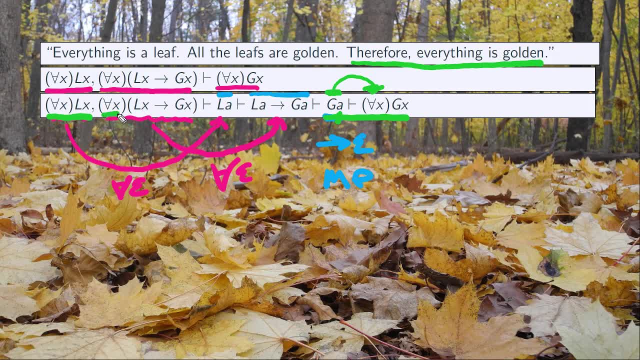 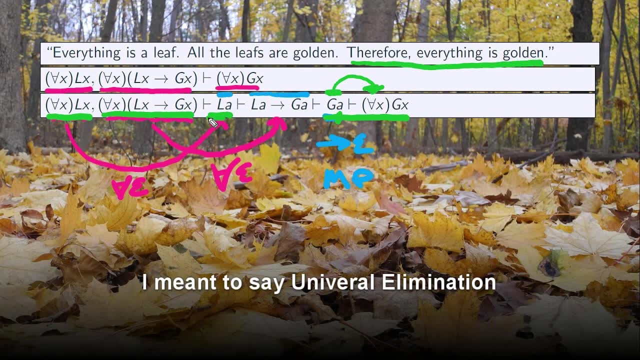 because this universally quantified lx and this universally quantified lx, then gx, we could have used universal introduction to drive b or c or d here, or we could have used it to drive a or b or c. 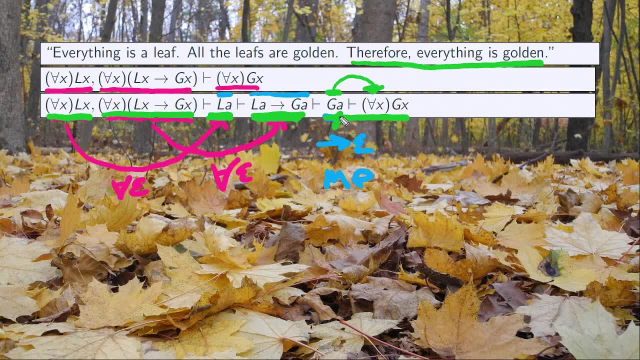 or d here. So given the fact that this ga right here, this a could have been any name and those names could refer to any item in the domain, it looks acceptable to use universal introduction. So we need restrictions. 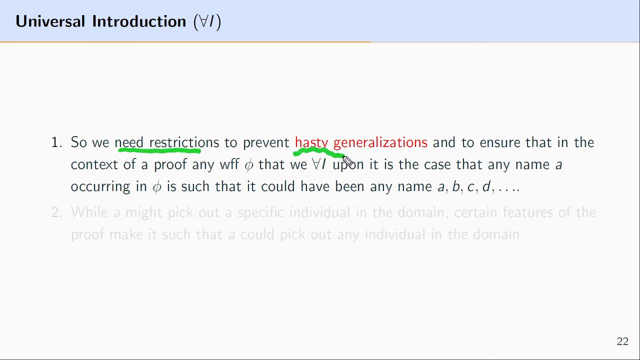 These restrictions are necessary to prevent hasty generalizations. That is, we put restrictions on when you can use universal introduction to ensure that on a proof where we have a well formed formula phi and we want to use universal introduction upon it. 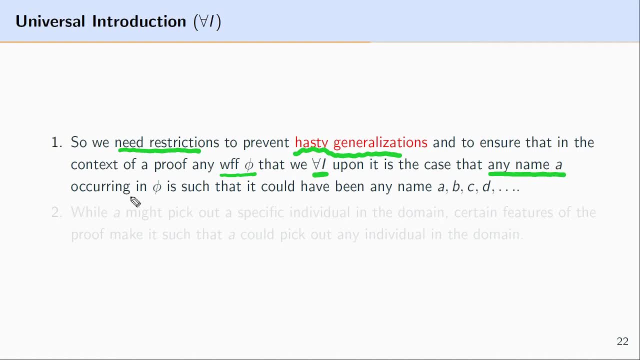 it's the case that for any name a occurring in that formula phi, it's such that that name a. so where is this name? this name a could have been any name: a or b or c or d. 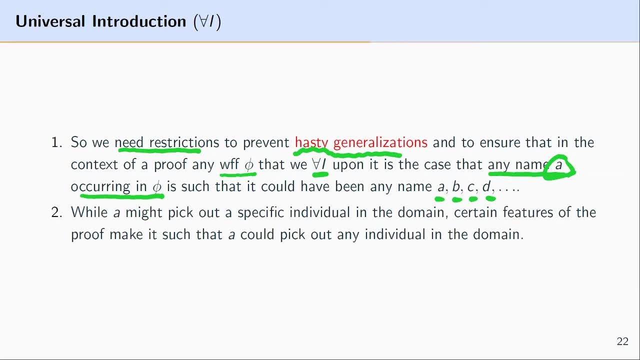 Another way of putting this is that, while a, the name a, might pick out a specific individual in the domain, certain features of the proof make it such that that a could have picked out any individual in the domain, That is. 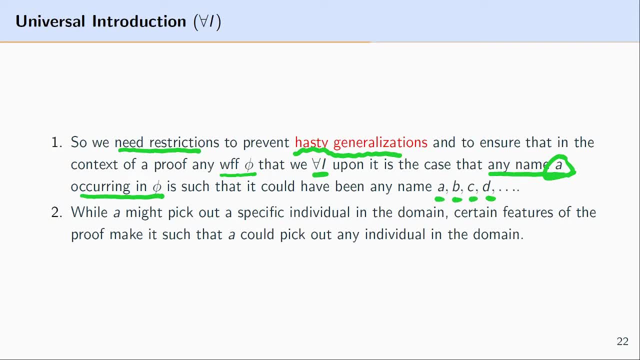 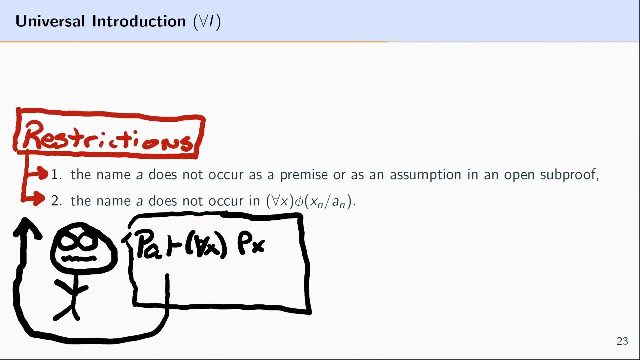 there's nothing intrinsic to the proof that makes a such that it picks out a specific individual. a could have instead picked out any of the items in the domain. So let's take a look at some of the restrictions associated with universal introduction. 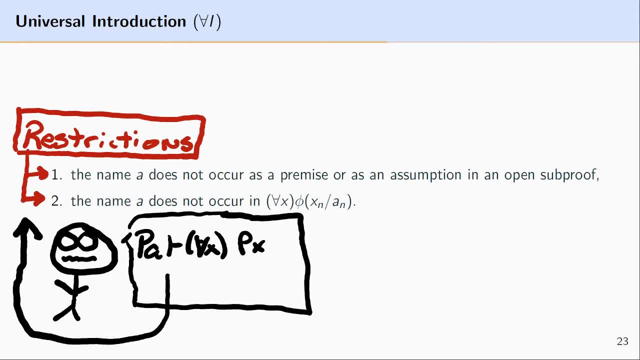 and then we'll walk through a number of examples showing you how to use this rule and how not to use this rule. So, whenever you're thinking about using universal introduction, so you're reasoning from something like p- a to for all x. 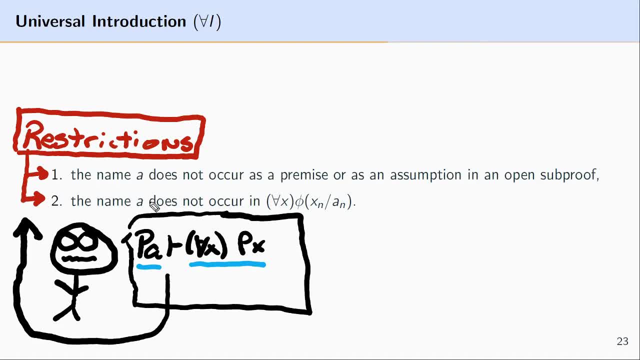 p x. you want to make sure that you don't violate either of the two restrictions. The first is that this a here that we're reasoning from it- cannot occur as a premise in a formula that's found in a premise. 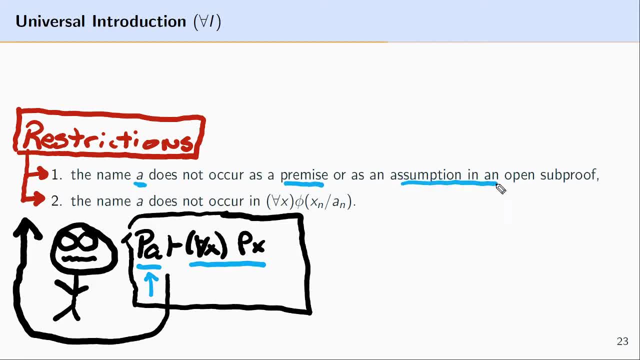 and it can't occur in an assumption that's found in an active or open sub proof. So, for example, if we reason to p a by making an assumption, we couldn't immediately write a x, p, x. This would be like saying: 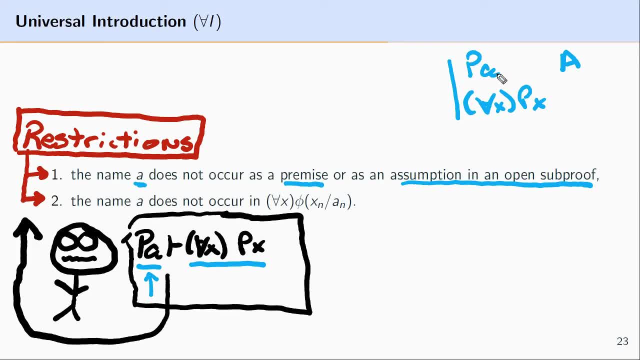 assume Alfred has a particular property, p, therefore everyone has that particular property. So the a that we're reasoning from cannot occur in a premise or an assumption in an open sub proof, and also the name a does not occur in the resulting universally quantified formula. 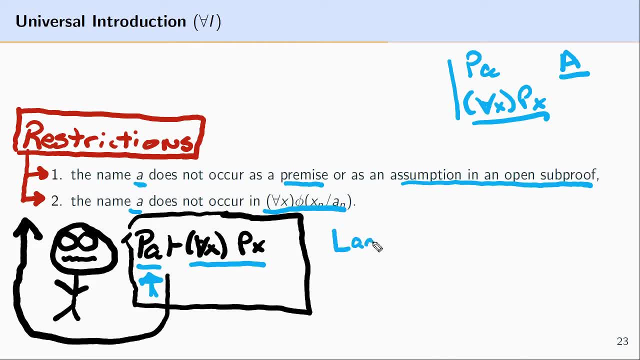 This would be something like, let's say, we said Alfred loves himself. We could reason, of course, to for all x, l, x, x. Assuming a is not found in as a premise or as an assumption in an open sub proof. 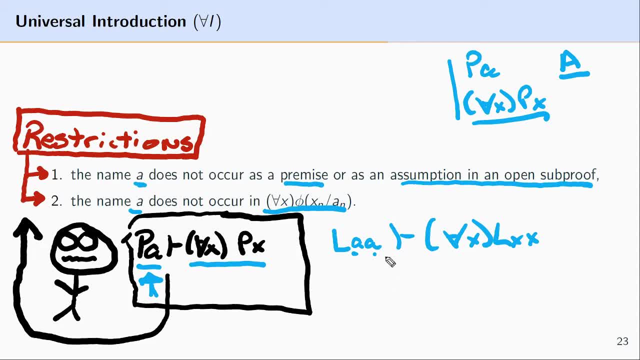 we could reason from a loves a or a loves him or herself to everyone loves themselves, But we couldn't reason from a particular individual loving themselves to for all x, l, x, a, That is, everyone loves one single individual. 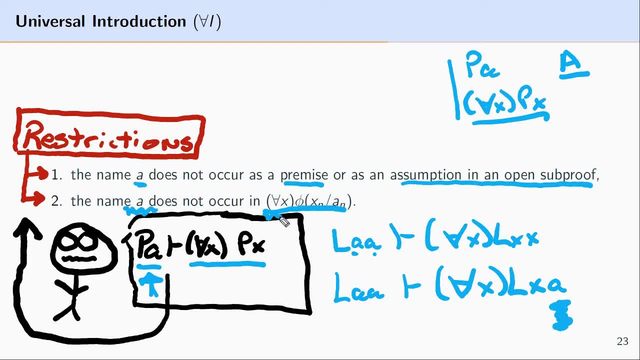 So we need to make sure that the name a does not occur in the resulting universally quantified formula. So, provided we adhere to these two restrictions, we can make use of. so now let's look at some examples. This is an example where 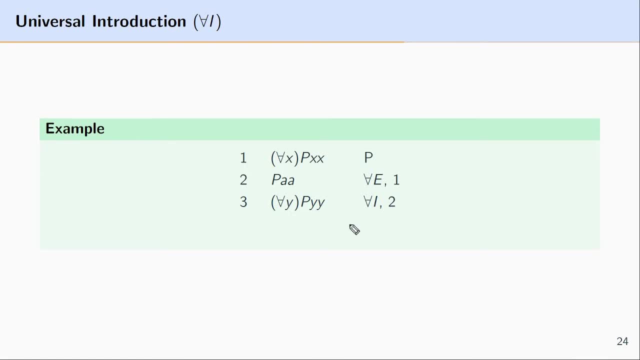 we make use of universal introduction and everything is fine and dandy. At line one, we have a premise which is a, x, p, x, x. At line two, we reason to p, a, a using universal elimination on line one. Then, at line three, we take line two. 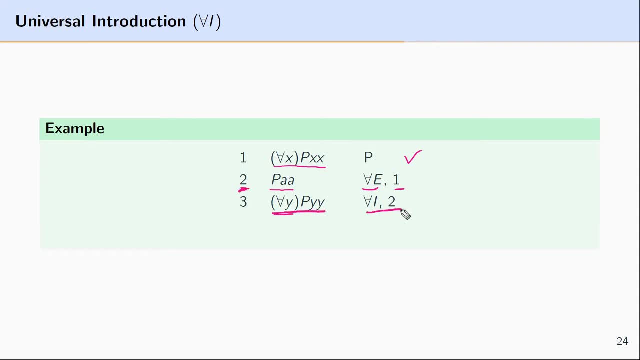 which is p, a, a, and make use of universal introduction on it Here. since a could have been b or c or d or e or any name, and those names could refer to every object in the domain, it's acceptable to make use of universal introduction. 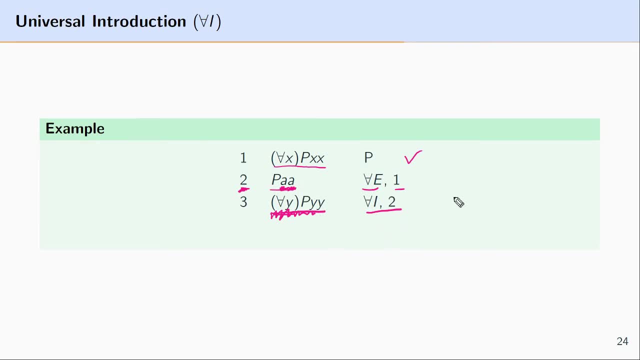 In other words, a does not occur in any premise or assumption in an active sub-proof and a is not found in the resulting formula. at line three We don't see any instance of the name a. This is another acceptable use of universal introduction. 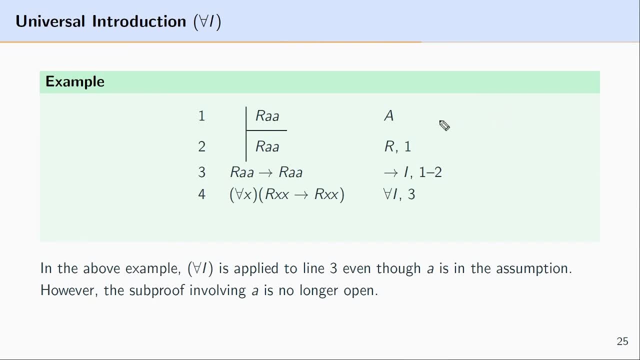 but it's fairly more involved. In this example, what occurs is: first there's an assumption of r, a, a, then, at line two, there's an instance of reiteration. At line three, we have a case of using conditional introduction, using the sub-proof. 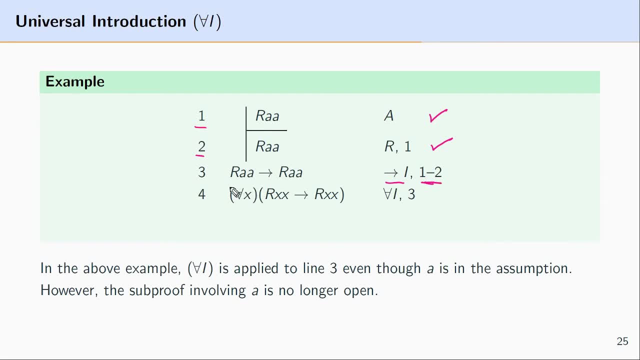 that begins at line one and ends at line two, and this allows us to reason to: if r a, then r a a. At line four, we make use of universal introduction, taking the entire formula at line three and replacing every instance of a 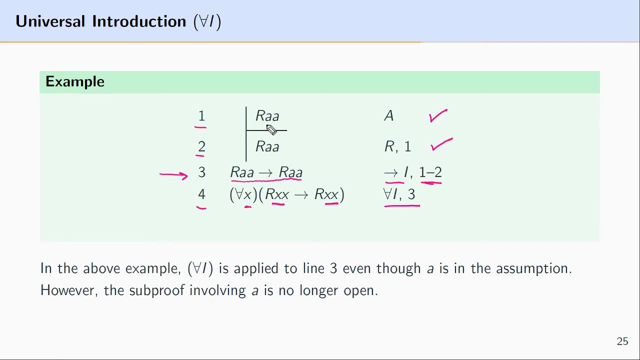 with the universally quantified x. You'll note, even though a is found in a sub-proof, this sub-proof is no longer active. That is, when we make use of conditional introduction at line three, this sub-proof is effectively closed. In addition, one of the things that you'll note is that 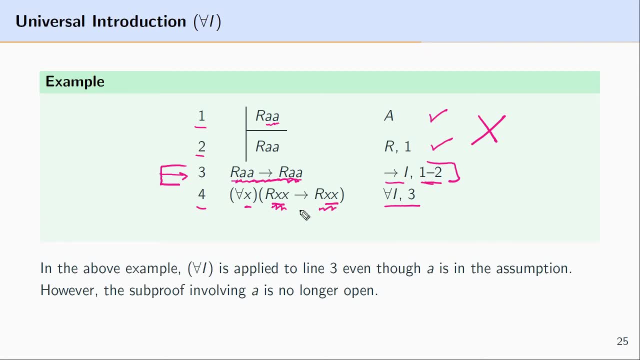 a is not found in the resulting formula, and so neither of the restrictions are violated. Furthermore, if you notice this, a could have been any formula. We could have assumed two b's up here, or c's or d's- any pair of names. 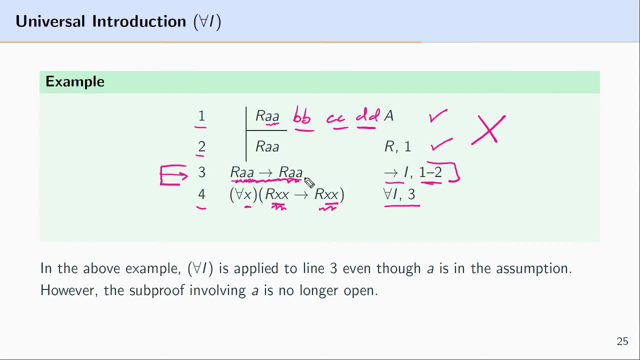 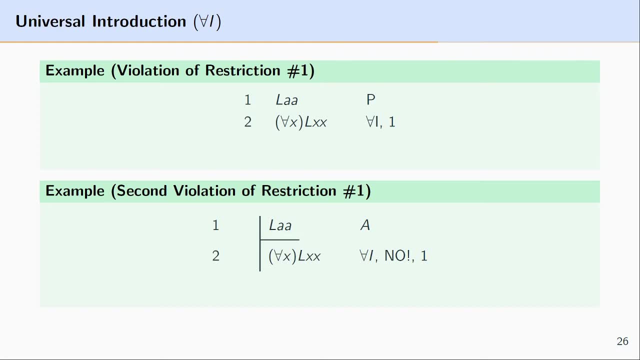 We could have derived r b b then r b b or r c c then r c c. Next, let's look at some violations of universal introduction, that is, cases where we use it incorrectly. First, if we had a formula like l, a, a,